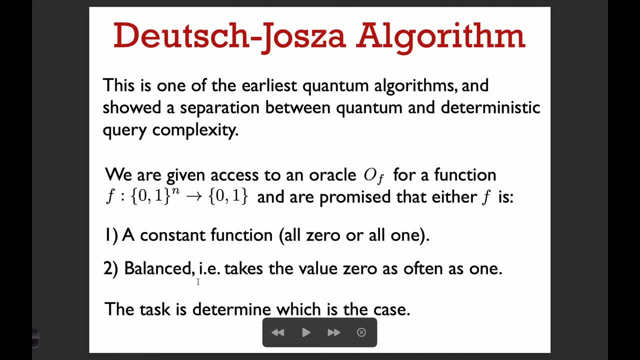 or f is balanced, so it takes on the value 0 as often as it takes on the value 1.. Okay, so we're given of, we're promised that f is in one of these cases and we want to use of. 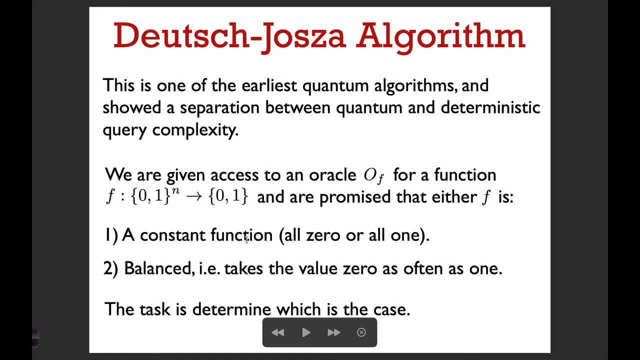 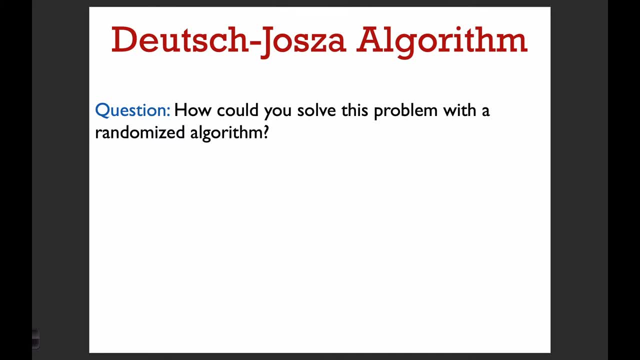 as few times as possible in order to determine which one is the case. okay, so before we get into quantum algorithm, let's first think about how would you solve this problem with a randomized algorithm? okay, so you can go ahead and pause the video and think about that for a second. I'll give the answer, right? 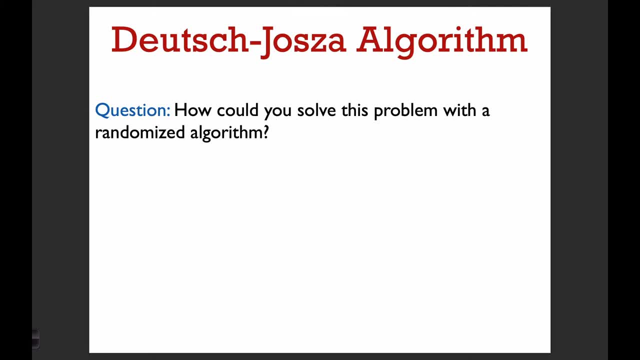 after this. okay, so this problem is actually very easy for a randomized algorithm. okay, the idea is that if the function is constant, then, of course, whatever we query, we're always going to see zero, we're always going to see one. but if the function is not constant, then if we just query a random X, the 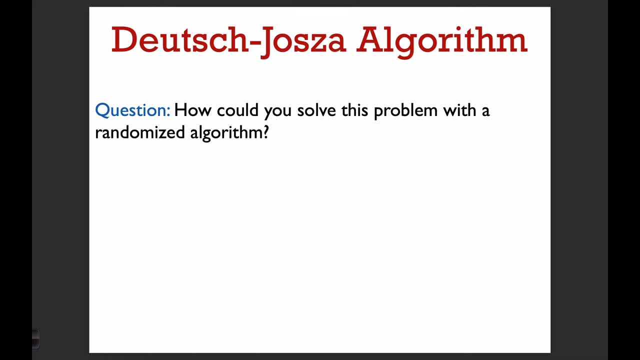 probability that we see zero is a half. the probability that we see one is a half. so if we just randomly query F at like you know ten different X's, with good probability you know with probably at least two thirds the function is balanced, we will see both the answer, zero and the answer. 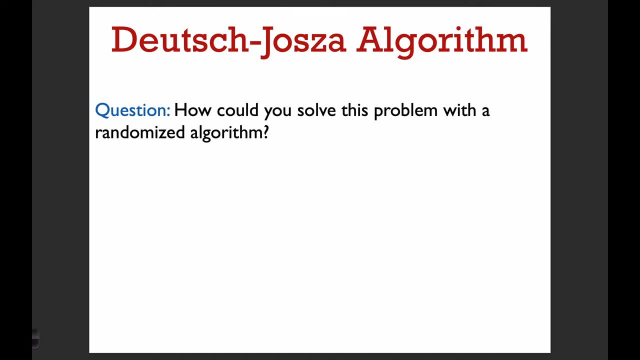 one, okay. and then we know that we must be in the balanced case. okay, so this problem can actually be solved, you know, with probability two-thirds, by a randomized algorithm just making a constant number of calls to the Oracle, okay. second question is: what is the probability that we can solve a random? 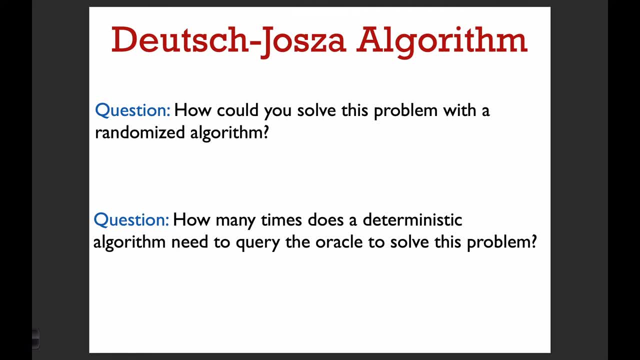 problem, okay. second question: how about for a deterministic algorithm? how many times does it need to query the Oracle to solve this problem? okay, so you can again pause the video and think about that for a minute. okay, so this problem is actually hard for a deterministic algorithm. so, in fact, a deterministic 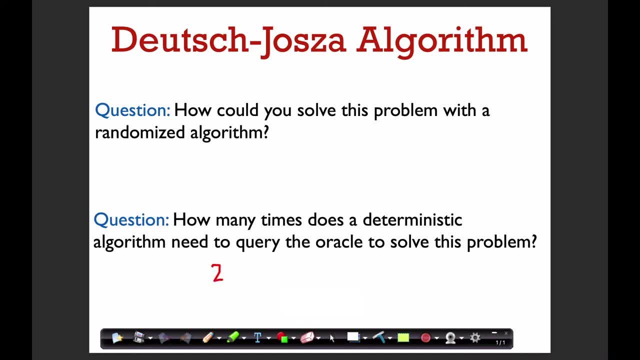 algorithm is going to have to query the Oracle- something like two to the n- over two times. okay, why is that? well, I can basically delve an adversary argument to to prove that. so say that the algorithm makes some query. I'm just going to answer that query with the value 0, okay. and even if I answer with the value 0 after 2 to the 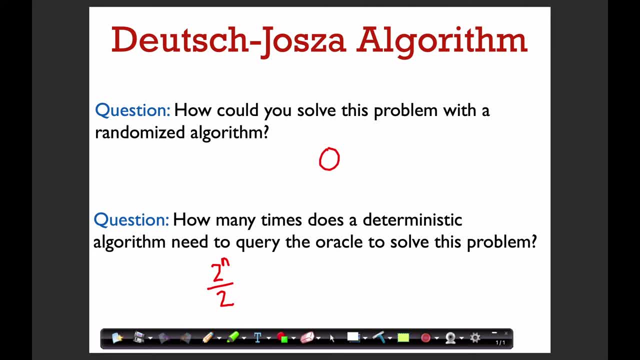 n over 2 many queries. the algorithm still can't decide with certainty whether the function is constant or not balanced. right, I can still choose how I answer the rest of the queries and to to make F correspond to a balanced function- you know, the all zero function- or to 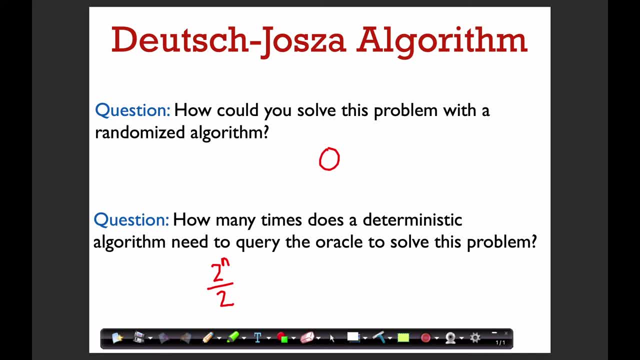 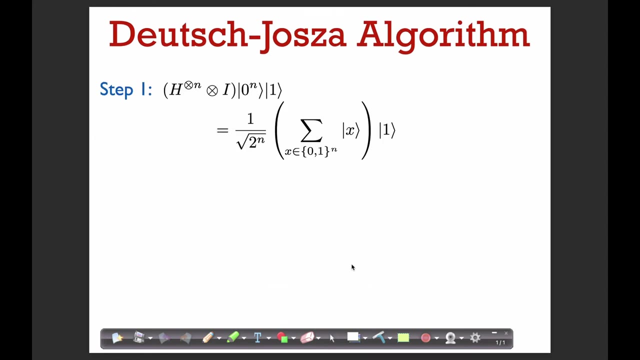 make it correspond to a, to a balanced function. okay, so that shows that you need at least to the in over to a queries to solve this problem with a deterministic algorithm. okay, so this problem is hard for classical deterministic algorithms. okay, so how does the Deutsch-Trosser algorithm work? 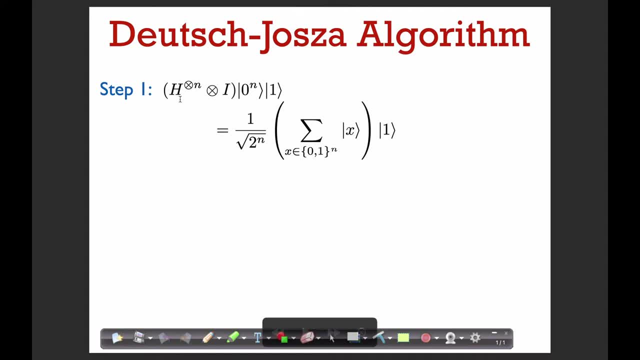 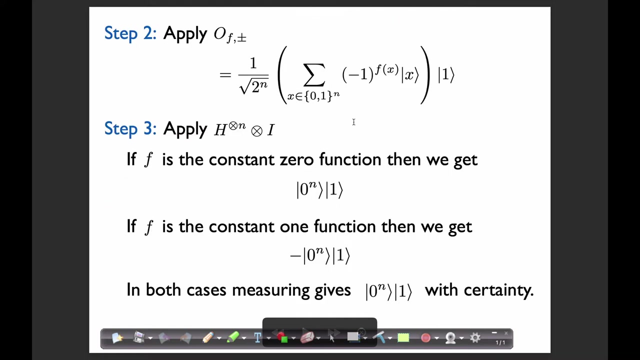 we start in the very typical way. we create uniform superposition on the first register, then we apply a phase oracle- okay, so that brings us to this state. and then we again apply, apply Hadamard on the first register- okay, so let's see what happens when we do that. okay, so first let's suppose that F is the 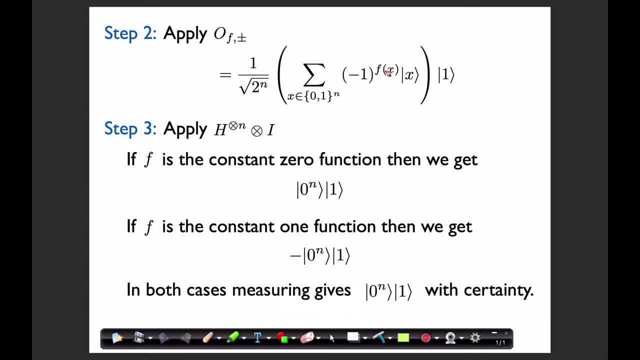 constant zero function. okay in that case. so f of X is always zero, so this phase here is always one. so that means that what we have here on the first register is just a uniform superposition over all X. okay, so then we apply Hadamard to that. it just maps us to the all zero string. 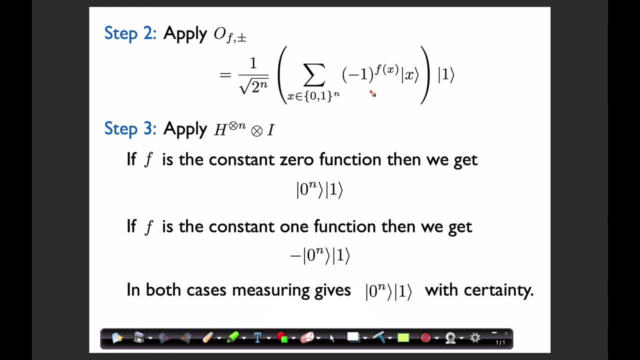 okay. so in the case where f is the constant function, at the end of this algorithm we're in the state 0 to the n tensor 1 with certainty. okay. similarly, if F is the constant one function, then this is always one and we basically get a global phase factor minus one. so after we apply Hadamard, we 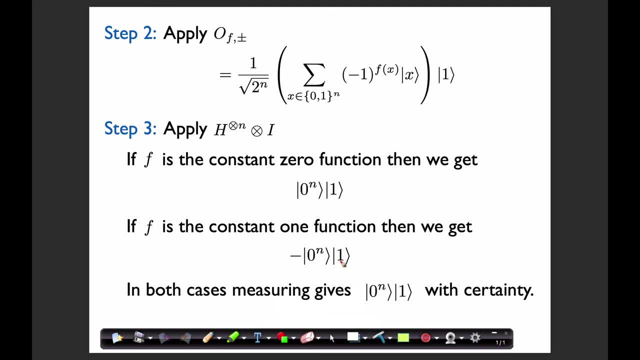 we're in the state minus 1 times 0 to the n tensor 1.. So in either case, when we measure we're going to get this state with certainty. Now let's consider what happens in the other case, when we're balanced. 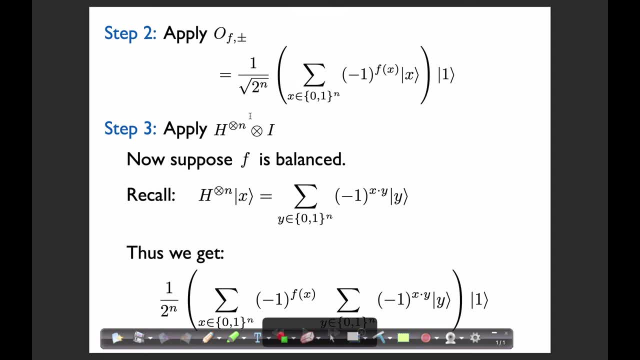 So we're in this state after step 2, and then we apply Hadamard to the first register. So recall what the Hadamard does to an arbitrary computational basis state. It does this, So we're just going to plug this in. 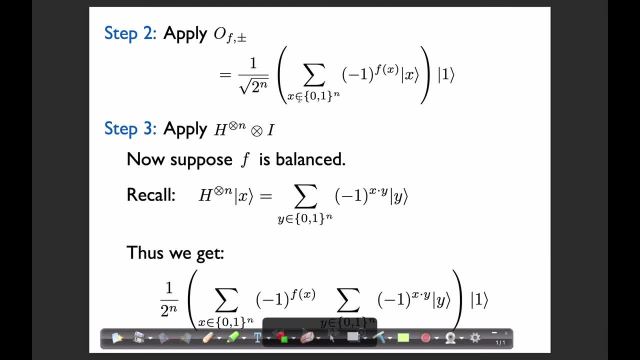 So what do we get when we apply Hadamard to the first register? We're going to get sum over x minus 1 to the f of x. And then what does Hadamard take x to? Well, it takes it to sum over all y. 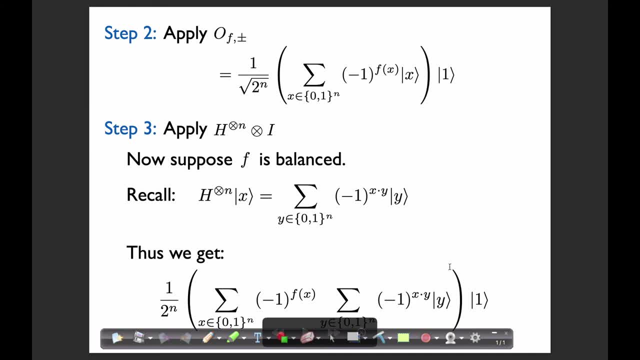 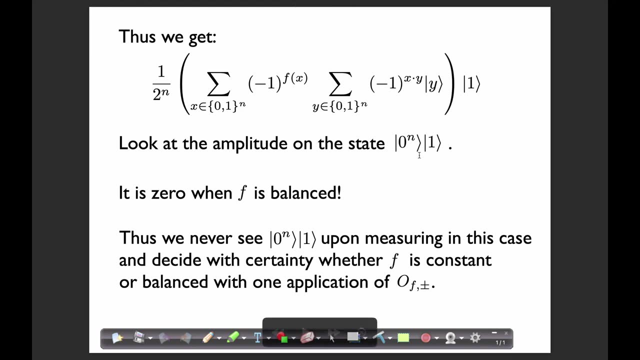 Minus 1 to the x dot y times y. OK, Now we don't need to work out what this entire state is. All we need to do is look at the amplitude on the state 0 to the n tensor 1.. Because we know, in the constant case, 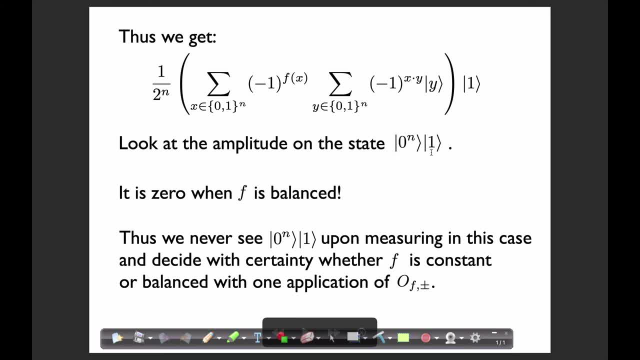 we're always going to end up in this state, So we just need to see And then balance. In this case, when we measure in the computational basis, what is the probability that we get this state OK? So think about the case where y is the all 0 string. 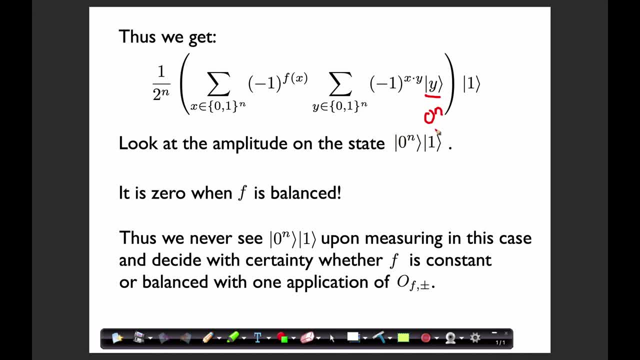 Because we want to see what the amplitude in front of this state is. OK, So when y is the all 0 string, then x dot y is always 0. OK, So this phase is always going to be 1.. OK.